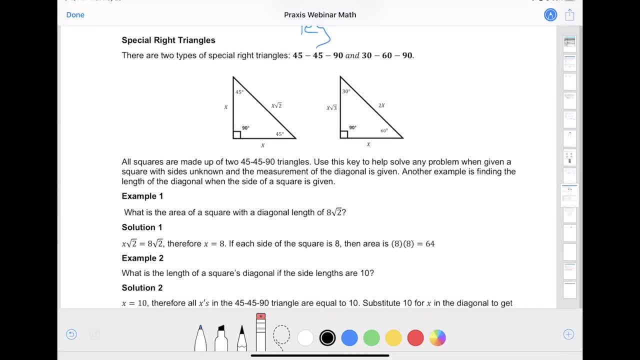 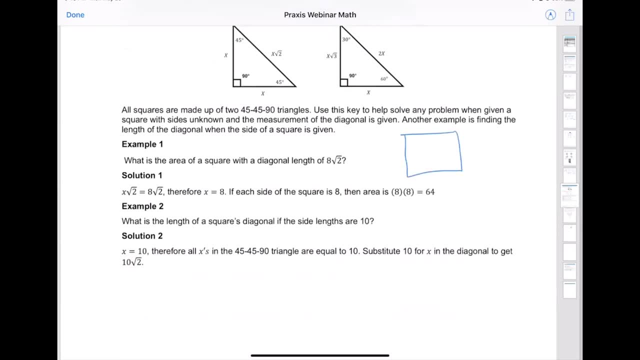 square with a diagonal length of eight square roots of two. So the square would look like this and the diagonal is just this right here. And if they tell me that this is eight square roots of two, what am I supposed to do with that? You can use the Pythagorean theorem, but you're going to waste your. 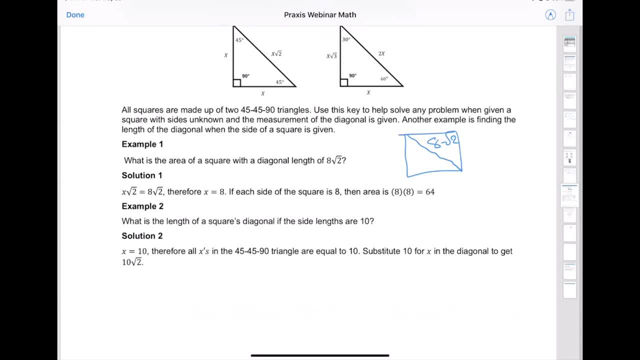 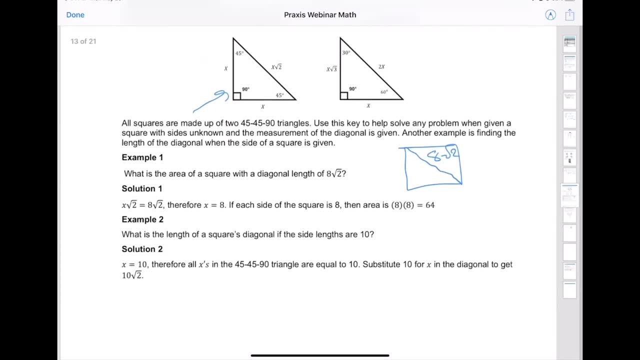 time It's too much. So what I'm going to do is I'm going to take a single triangle is supposed to be like this one right here. I'm sorry, every square has a triangle that looks like this right here. Then we're going to go ahead and match it up to this eight square roots of two. So if I go ahead and draw it right next to it, I'm going to draw that triangle with eight square roots of two. OK, So look at the triangle that you have, Sorry. 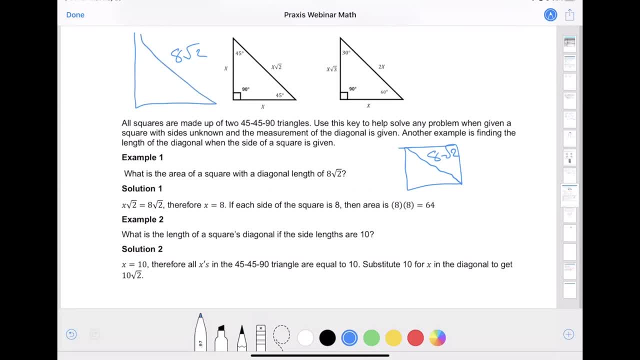 Look at the triangle that they give you with the eight square roots of two here, And I've got nothing on the legs where this is X and X. But I have something right here. If I were to take this triangle and put it right on top of here, this eight square roots of two would land right on top of that X. You could say that they were equal to each other. So then, if I see that it's eight square roots of two is equal to X square roots of two, Well, if the eight's here and that's an X, you know that the 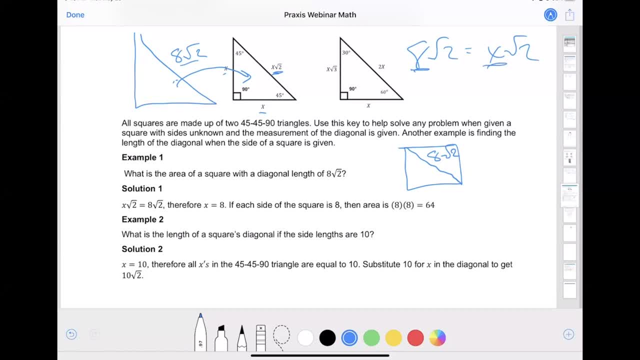 missing missing value has to be eight. So X equals eight. So that means in this square the dimensions of the square are eight by eight. Since they want the area of the square, be careful, it's a two part question. Since they want the area, you have to find the side lengths and then multiply those side lengths together. If you have eight and eight, just like you do here, that's going to be 64 and that's going to give you the area of that square. The next: 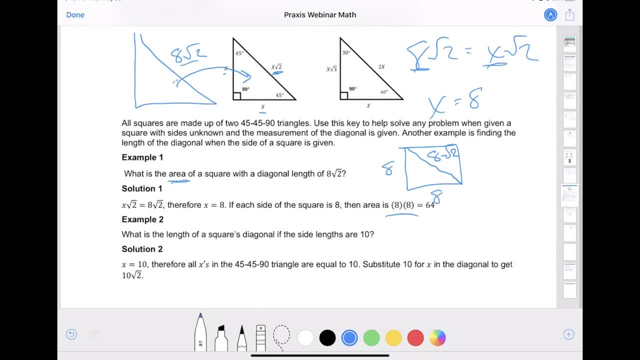 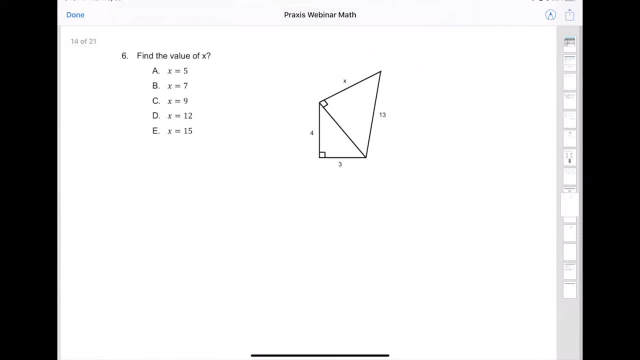 example Just shows you, when they give you the legs, how to get the hypotenuse. But this problem: here we see that we have two triangles, specifically two right triangles, and I'm given four and three and X and 13.. Well, if I figure this triangle out first, that'll give me the value here, and then I can use that to find the second one. So it's a two parter. 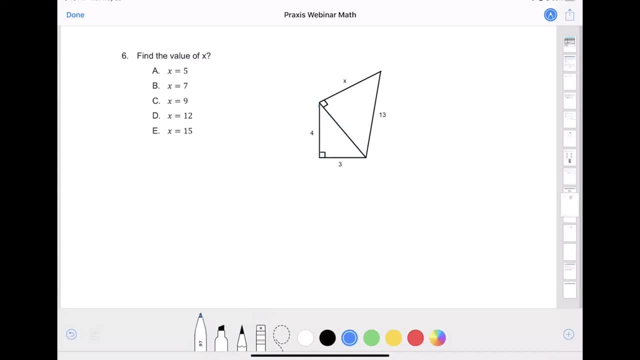 So, using my Pythagorean theorem, AB is always the legs, C is the hypotenuse. Hypotenuse is always opposite of the right angle. So I want to do, for let's do this: A squared plus B squared equals C squared. So if I do four squared and three squared, it has to equal my C squared. 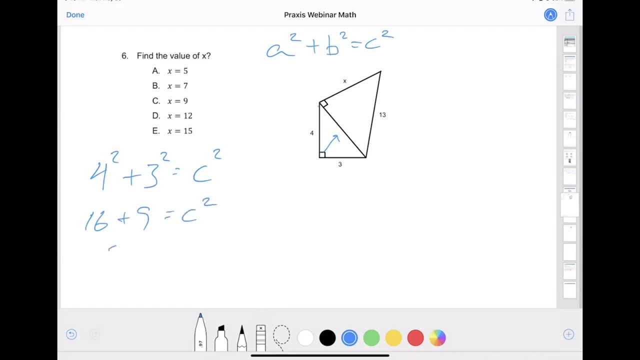 16 plus nine equals C squared gives me 25 is equal to C squared. that squared is there. C's got to be completely by itself. how do I get rid of it? the opposite of squaring something is square rooting. so I want to square root both values and I get 5 is equal to C. 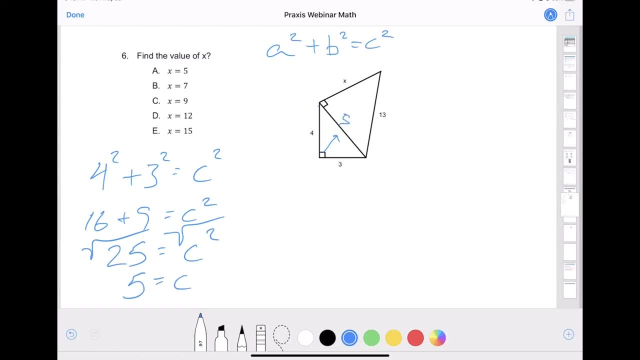 well, that means that 5 belongs- oops, 5 belongs- in this spot right here. so now I take the same thing and do it again for this big triangle. I take my leg. in my leg I'm gonna have x squared plus 5 squared equals 13 squared, and then just 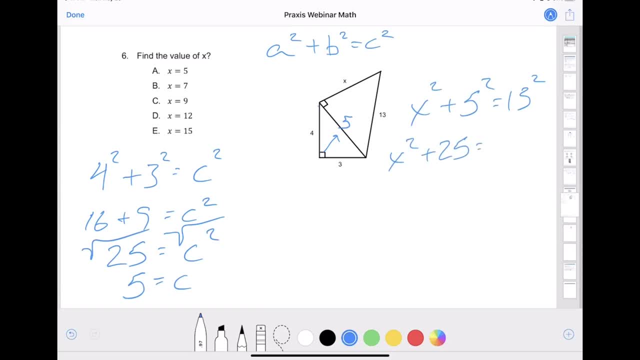 run it right down and then this time, you see, it doesn't work out like the other one. we have to bring our value over x, squared is equal to 144 and then, finally, square root x is equal to 12. for this type of problem, you know, you got to put the work. 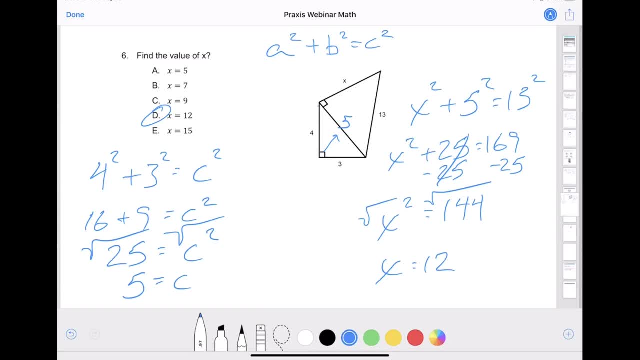 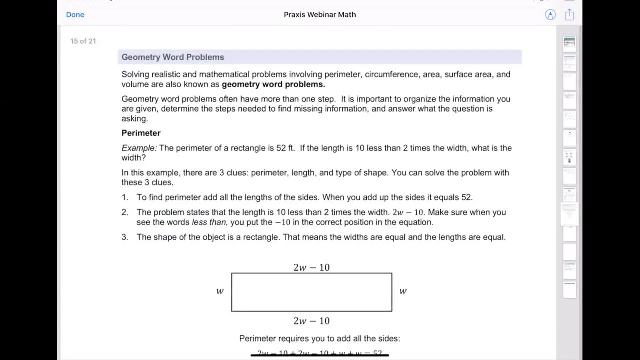 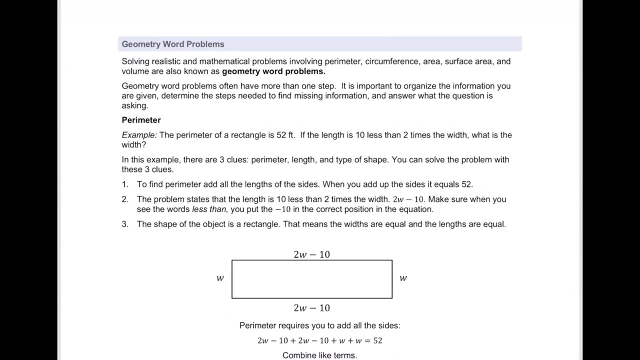 in, but as you, as you practice these over and over, though, they'll come to you right away and you'll just be able to breeze right through it, okay. geometry word problems. be careful on the geometry word problems, because there's a lot of terminology that goes into it and you have to be- you have to be aware of what. 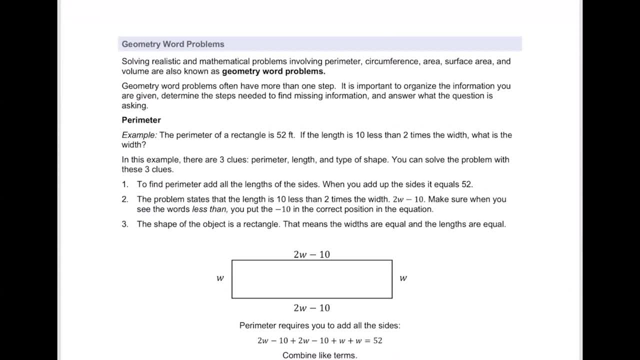 it is that they're talking about especially the perimeter, circumference area and surface area. so I'm going to go into this. one for perimeter. perimeter of a rectangle is 52. if the length is 10, less than 2 times the width, what's the width? and so, as I 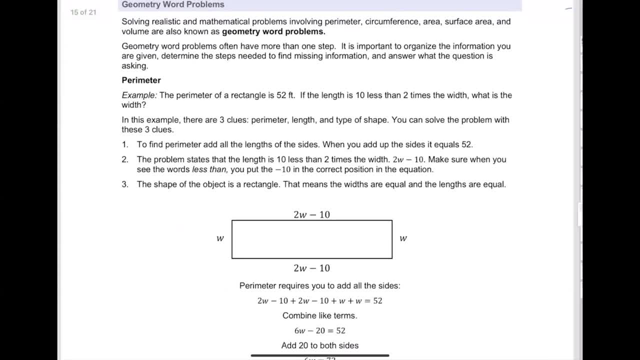 go into this. I look at the problem and I and I pick out what it is that I need to know. we're dealing with perimeter. if they're telling you what the perimeter is, chances are you're gonna have to use perimeter to solve this in some way. 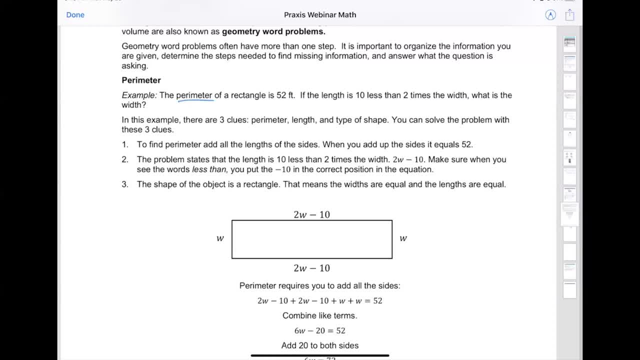 shape or form, and there's my value, 52, but also it's a rectangle. that's also important, because if you're going to have to solve this in some way, shape or form, and there's my value, 52, but also it's a rectangle, that's also important- the 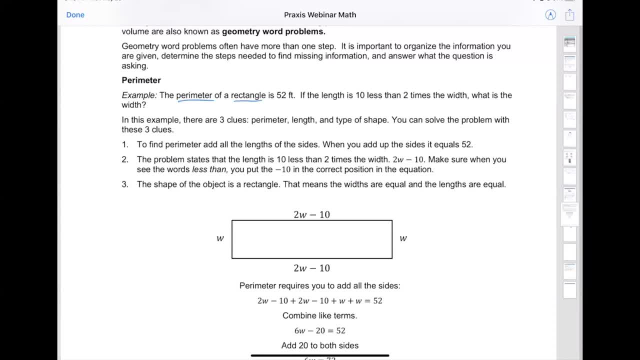 because we know special properties about rectangles. so first thing I'm going to do is I'm going to draw a rectangle. draw a rectangle on my, on my, my paper, okay, so once I have that rectangle, I go ahead and start filling in the information. it says: 10 less than two times width. be careful with this because 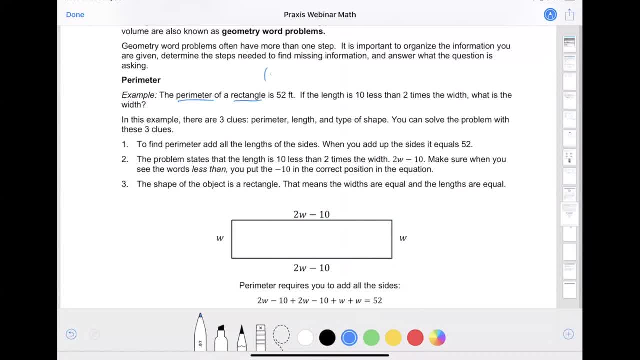 as we read it, some people may just say 10, less than two times width, and when we we do that, we're actually wrong because of this: less than, with less than and with fewer than, these are the only times in math with um and it deals with subtraction. that, as you read it, you. 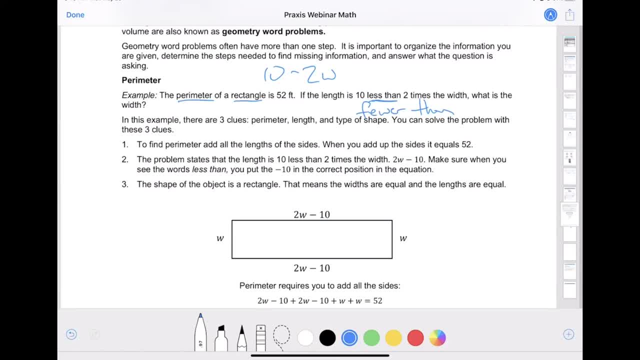 write it backwards. so that's why this is 2w minus 10 and this one is incorrect. so watch your less than and watch your viewer then, because i can tell you that there's a high percentage chance that you will see this on the exam because of the way that this is done. so, now that i know that, 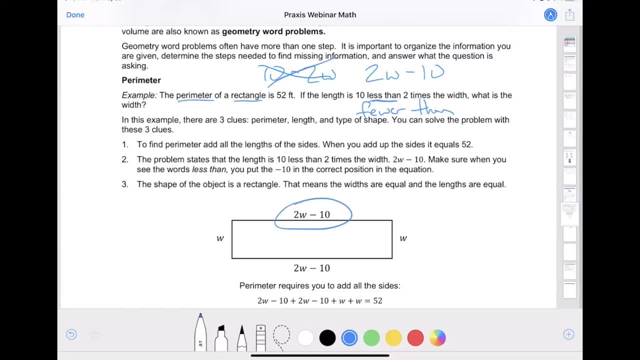 that's one of the lengths. i put the 2w minus 10 here because it's a rectangle. we know opposite sides are the same, so that's why the 2w minus 10 is there as well. and then w goes on for the width. 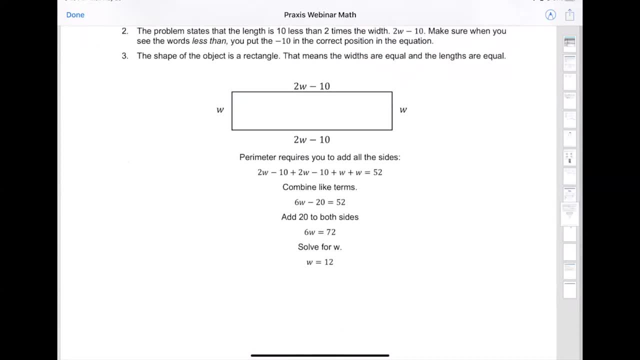 and so now remember it said, perimeter is equal to 52. well, how do i incorporate that in solving this problem? perimeter means to add all sides, so literally add all the sides that you have and you'll get this equation here. another way to do it is group. 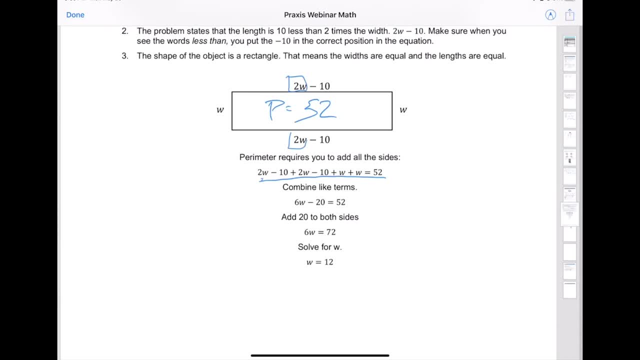 it out. i see all my w's are right here. so how many w's do you have? we'll have two here. one here makes three, two more make five, one more make six. i've got six w, and then what's left are my negative ten and negative ten, and that gives me negative ten. 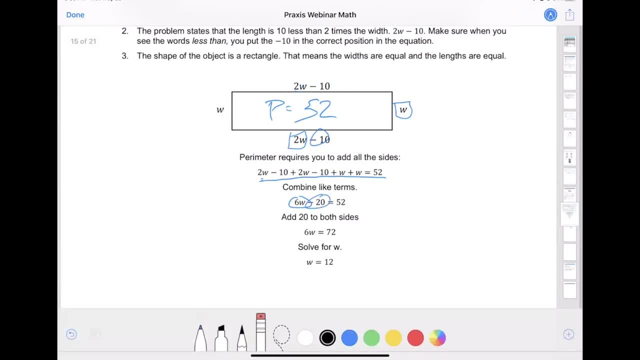 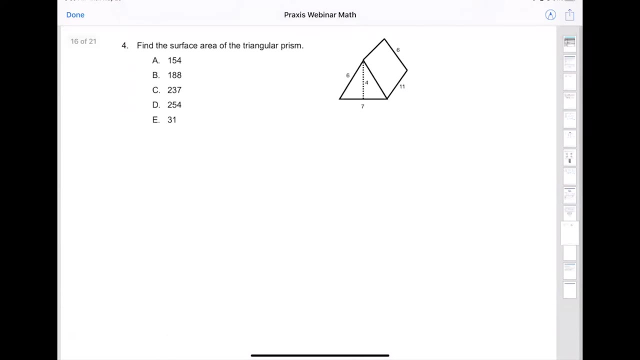 negative 20 right there just kind of falls right into place, okay, and then from there solve it just algebra. the most important part is getting this rectangle with the right dimensions and then, knowing that it's perimeter, and just go right from there, solve it real easy, okay. the next one we have here is talking about surface area. what is the surface area of this? 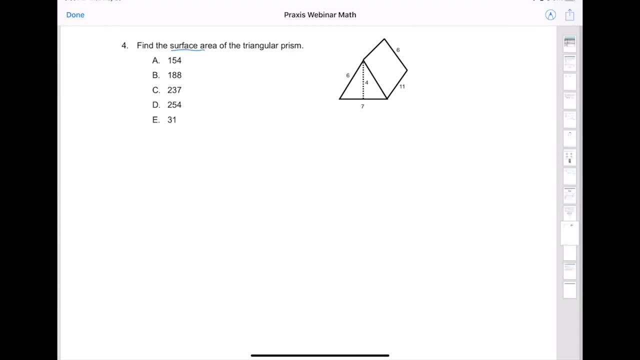 triangular prism, and so this may take a little time. but the best way to do this is to unfold the object, so to speak, and you make what's called a net. so I'm going to go ahead and the base or the bottom pretend this is a tent, so this would be the floor. there's a rectangle here and it's the floor. 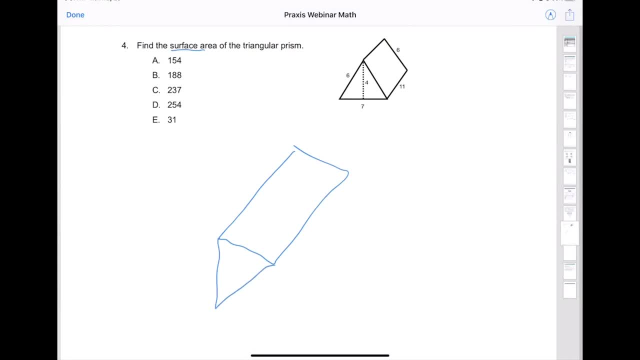 and then here's that first triangle, you see, but because it's a prism, it has two of the same bases. so there's one there. then I'm just going to unfold it so that I'm left with the right dimensions, and then I'm going to go ahead and solve it right from there. solve it. 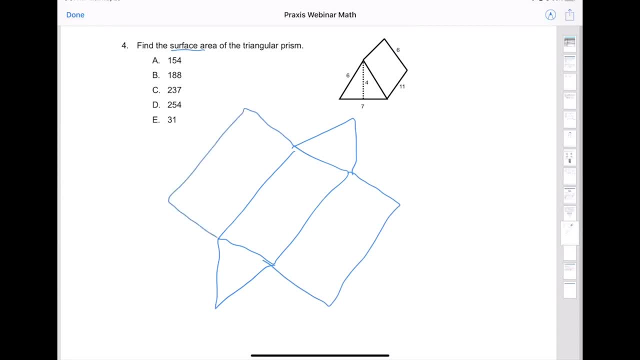 with a rectangle here and a rectangle here. so if I flatten that object out, that's what it would look like in two dimensions. then put all your, all your, your measurements. this is 11 and then, as we see how the six was here, that also means there was a six here. so that's a six, this is a seven, this is. 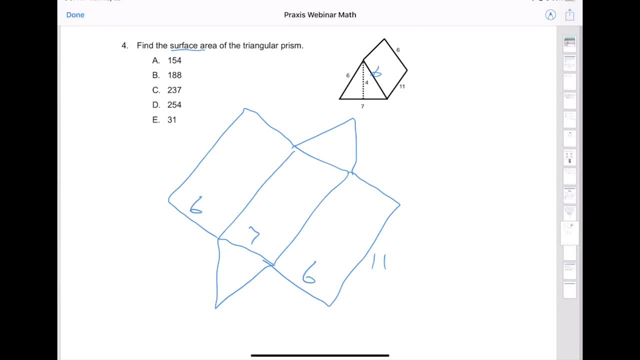 a six. and then for my triangle you have this: this is called the altitude and this is four. so now what I want to do is I want to see this as- and just look at the big picture here- surface areas. when we add up the areas of all sides, there are one, two, three, four, five sides in this shape. if 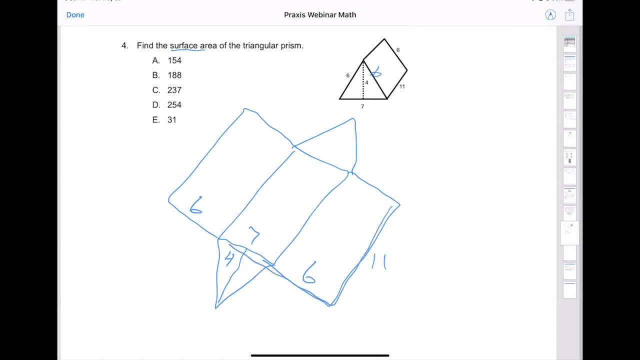 I look at this right here. so if I see this as one big rectangle, okay, then add these bottom dimensions and then multiply it by the 11. so if you can see that, that will help you tremendously. so let's do 6 and 6 is 12 plus 7 is going to give us 19, right, so we have 19. excuse me, I have 19 times. 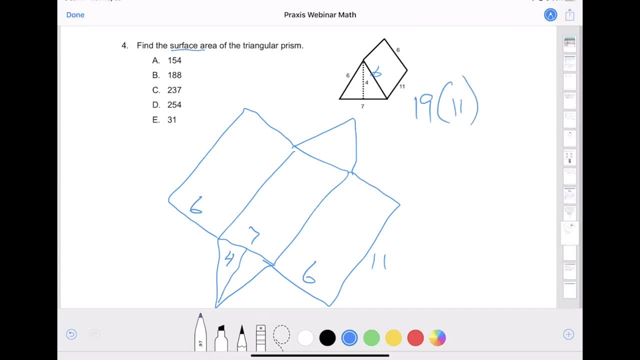 11, and then that's going to take care of all those sides. and now I got to figure out what this triangle is. well, area of a triangle is going to be 1 half base times height. base is 7, height is 4, so I'm going to do 1 half base is 7 times 4, but I have two triangles here. there's two sides, so 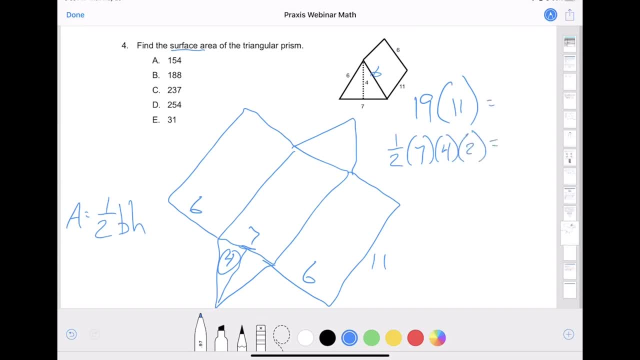 multiply that by 2, so, as you do the math real quick, you get 209 for the big rectangle part and then you get 28 for for the two faces. add them up, then you have 237. the answer is C. so if you can visualize and unfold your, 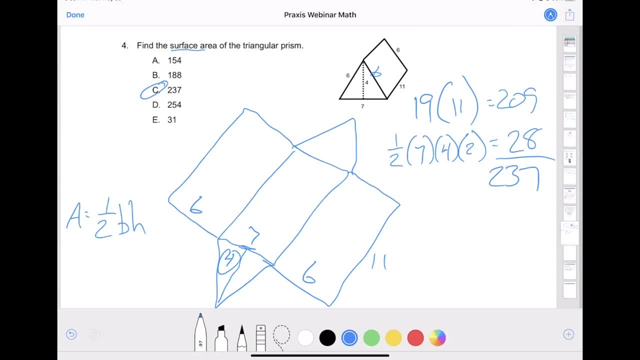 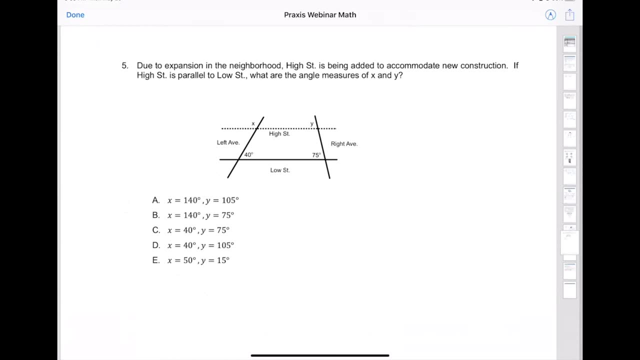 three-dimensional objects into what's called a net, you will see that it's much easier to go ahead and find that surface area onto some more with angles and different measurements. here you can see that these are parallel lines: this line, this line and this line. any time a line goes through a parallel line is called a transversal. so what? 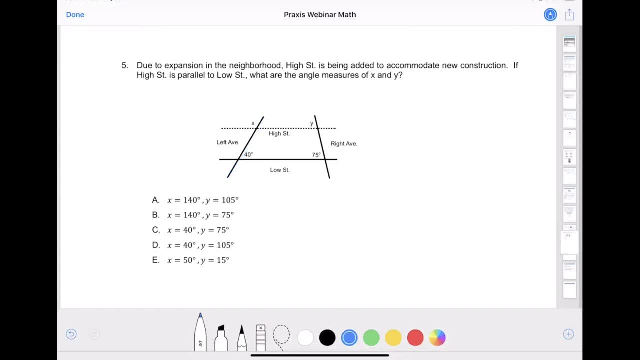 happens is something special where, if I were to box out these intersections, they are exactly the same. as long as they're on the same transversal, they're exactly the same. so when they want me to find out what these variables are, if I were to take this intersection, pick it up and drop it. 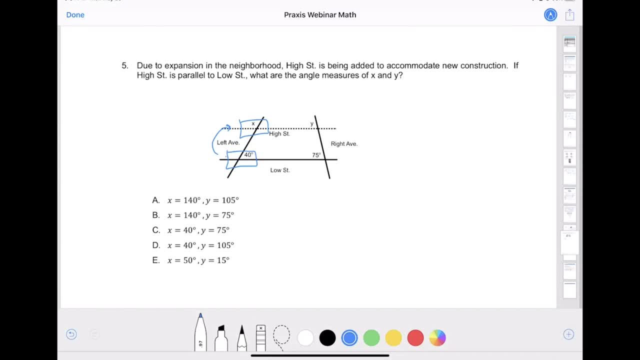 right onto here. the corresponding parts would go ahead and equal each other, or just think of it like this: go to the upper left hand quadrant, so our upper left hand. so Up Left is this one, Up Left is this one. this one has a value. it's x. that means that one is X and same here, that's 40. so that has to. 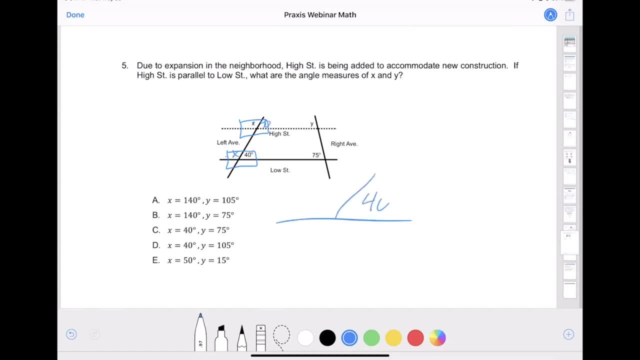 be 40.. so it's looking like this: right here we have a 40 and an X here. well, we know that straight lines are equal to 180 degrees, and if it takes 40 degrees to get from here to here, how many degrees does it take to get from here to here? Well, if the total is 180, subtract my 40, then that gives.